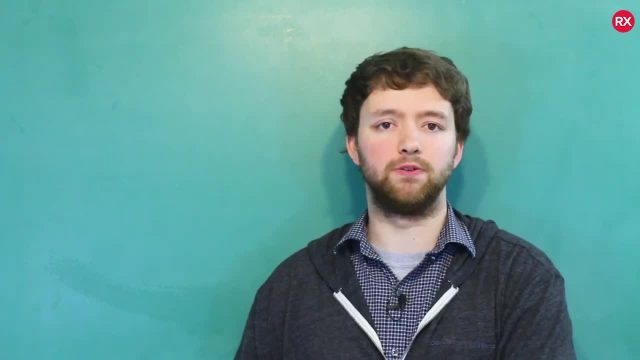 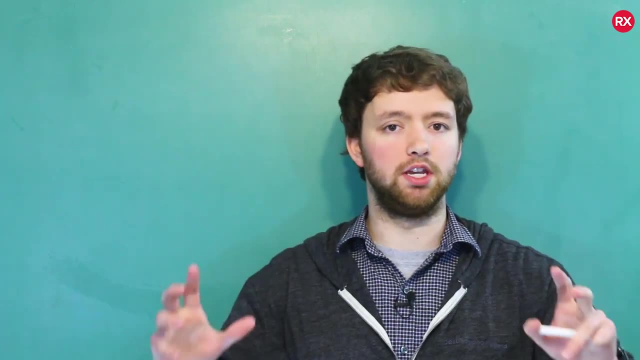 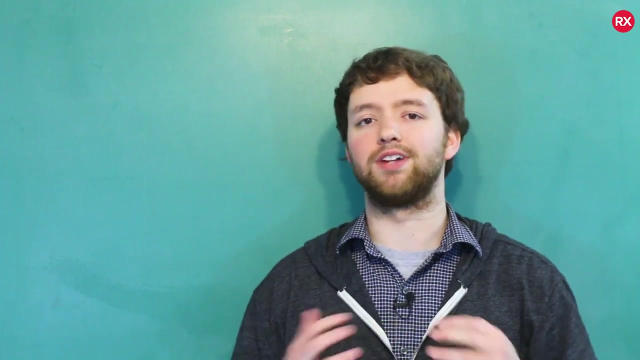 So C++ is a concept inside of a programming language which C did not have in C++ introduced And it really set the foundation for a lot of the other programming languages: Java, C, Sharp and basically all the C-like programming languages. all have the object-oriented programming component. 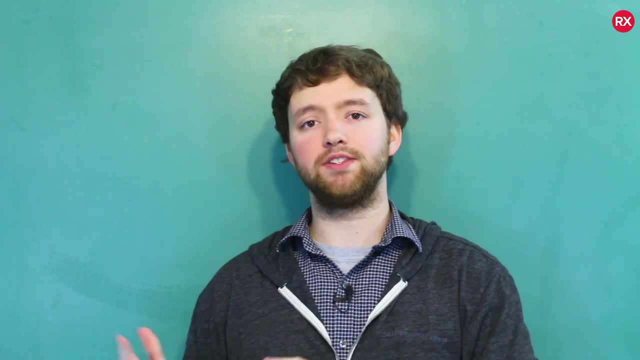 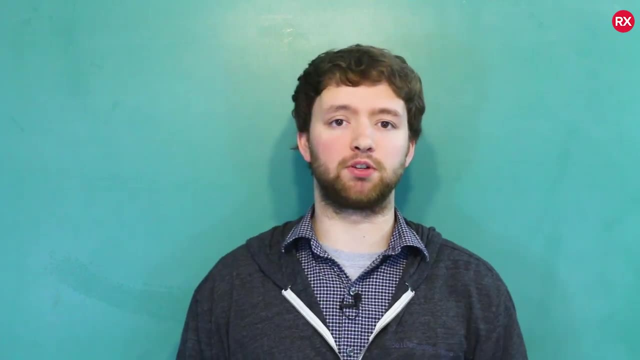 in them. So learning this stuff is not just for C++, it's for everything. But the way you do it in C++ is definitely a little bit different than the way you would do it in C, Sharp or Java. So we're going to talk about C++, object-oriented programming. It's not just going to be general concepts that 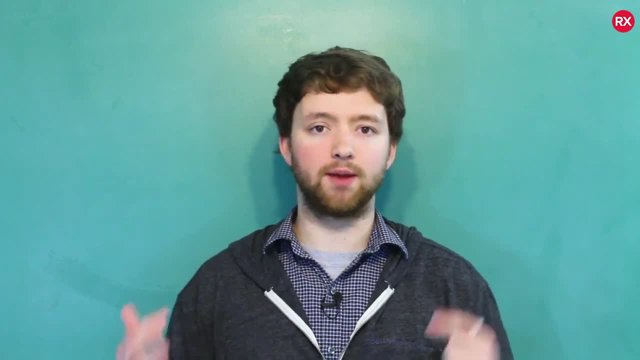 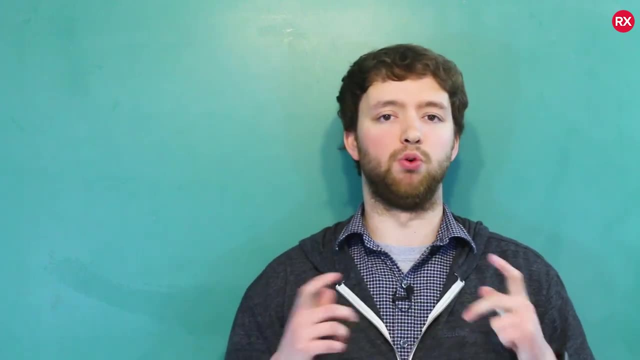 you could apply to anything. We're going to get really specific, so I'm excited. hope you guys are as well. So there's a lot of info about object-oriented programming, but I think one of the big struggles people have with it is the why. Why do you need object-oriented programming? And that's. 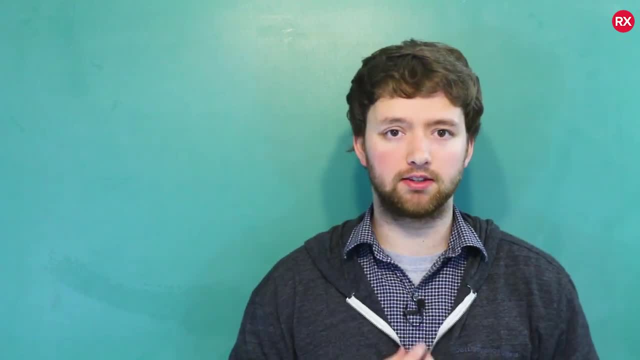 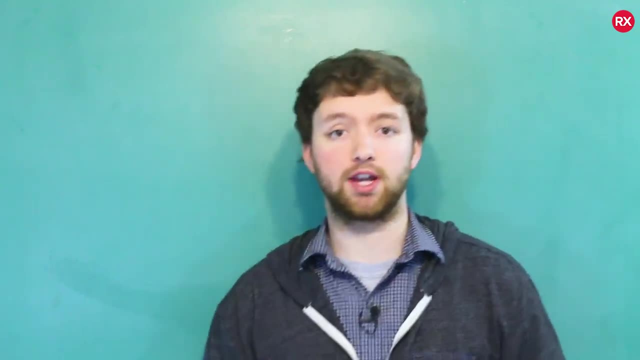 one of my big goals that I hope to basically explain to you guys. But first, before we get into the why, let's talk about the. what Object-oriented programming is based on the concept of classes and objects. Here we have a class And we define a class in code. It basically defines a structure. It's the blueprint. 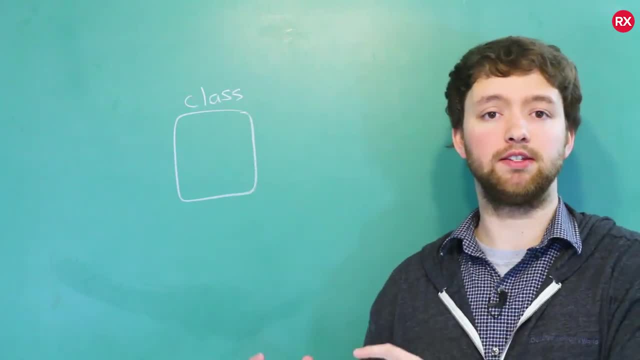 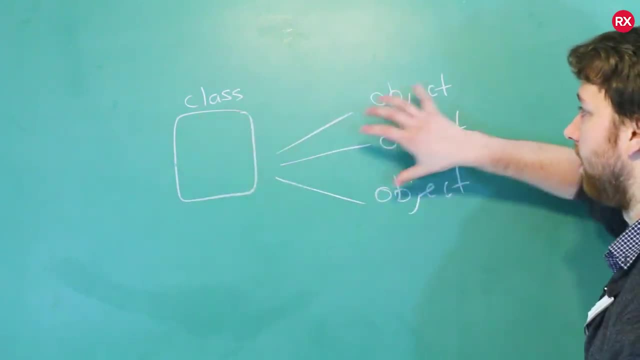 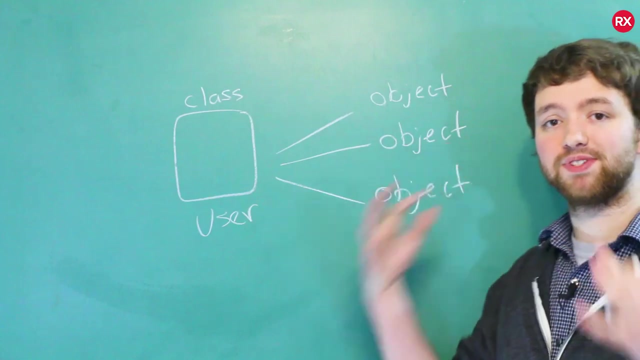 It's the cookie cutter, And we can use that cookie cutter to make many instances, And these instances are known as objects Like so. So class is used to define an object. This is the structure. Think of this being like a user And each object being a specific user. 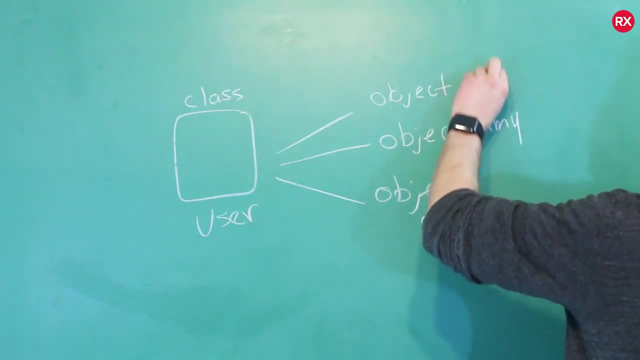 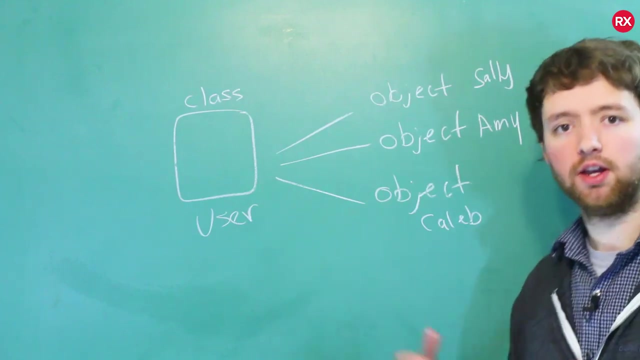 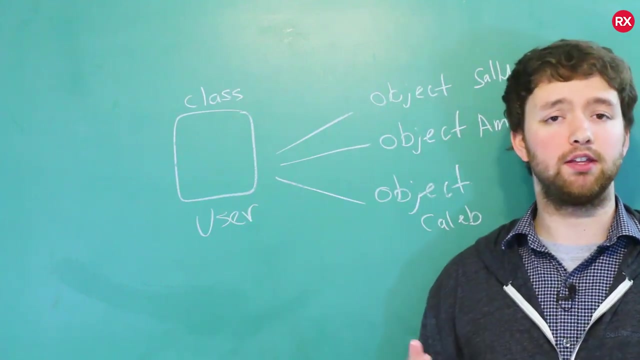 So we might have Caleb, Amy and Sally Or whatever the names are, It doesn't really matter, Just users. Now why do we structure things this way? Well, because most applications we do are built around data, And data is a very general term that can mean anything. 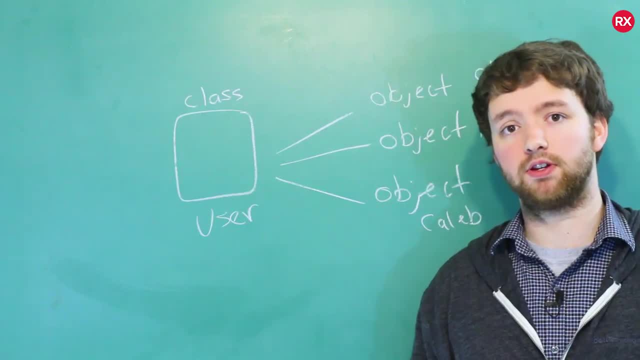 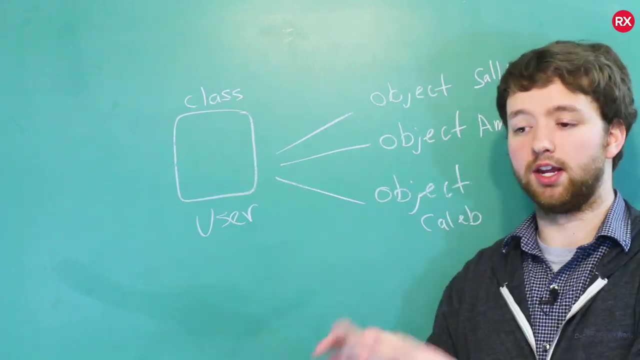 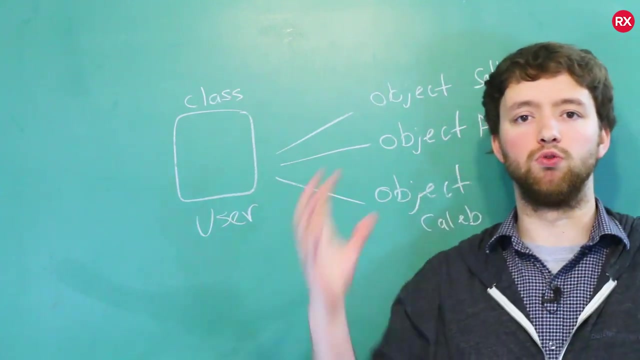 But usually our applications are data-driven applications, So we basically can describe data or real-life things using objects. If someone creates an account on our application or creates a user, then we can describe that as an object. It's basically a way to group and 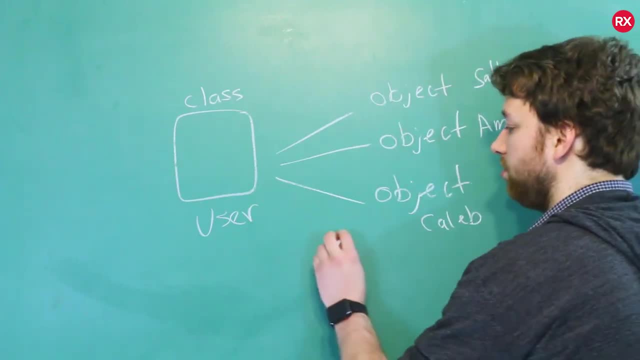 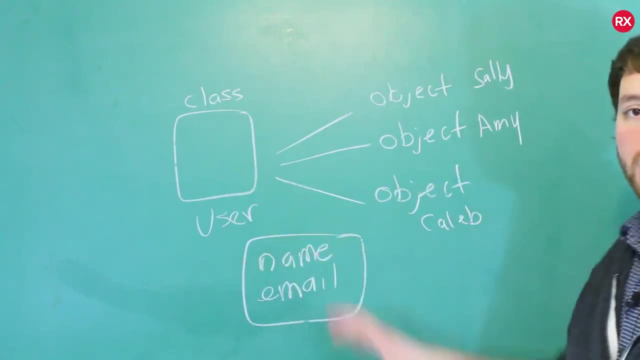 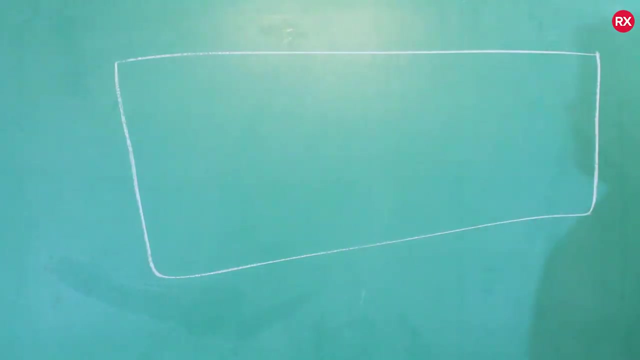 organize information and keep things organized. So within one user we can have the person's name, their email and so forth, But it's all grouped within one object, so it stays nice and organized. Another way you can think about object-oriented programming is a table. So no, not like a dinner. 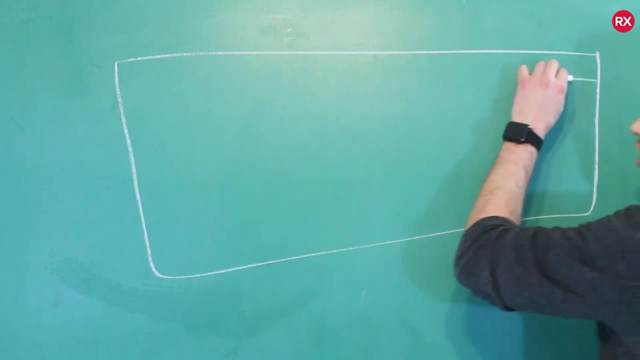 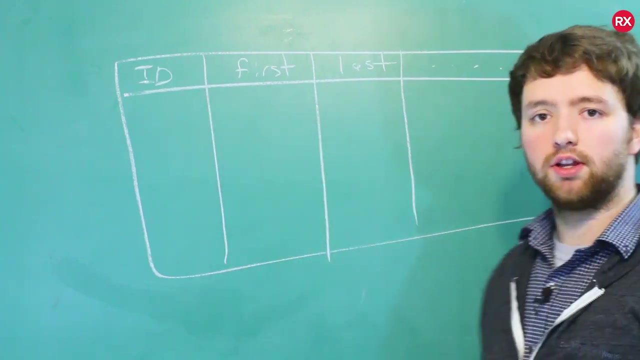 table. We're talking like an excel table or a database table. Usually we have columns, So we might have a column for their ID, their first name and their last name. Well, these column headers consider them to be the class. It defines the structure, And then each individual row is like an object. 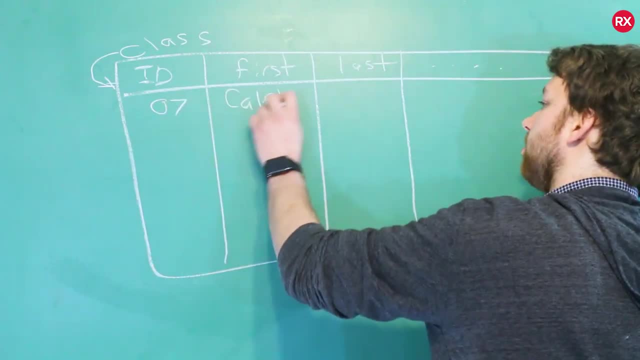 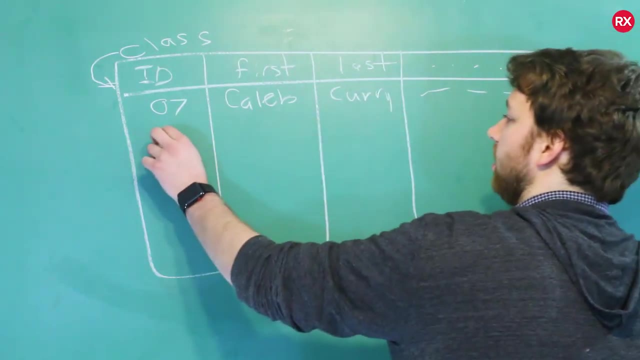 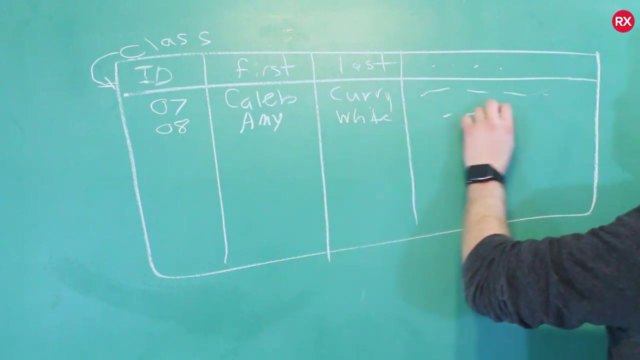 So this person might have the ID of seven, have the name Caleb, last name Curry and then some other information. Here is one object. We can have another object with the ID of eight. This person can be Amy, last name White, and so forth. So once again the columns are like: the class defines the structure. 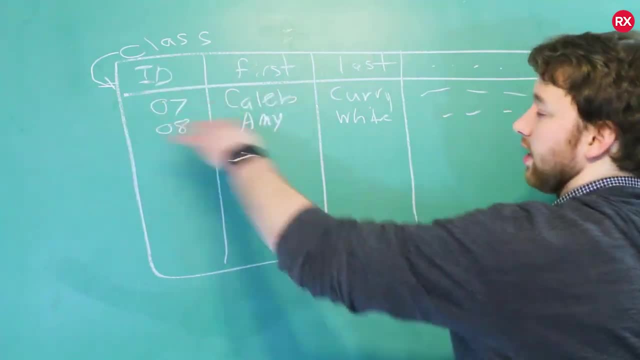 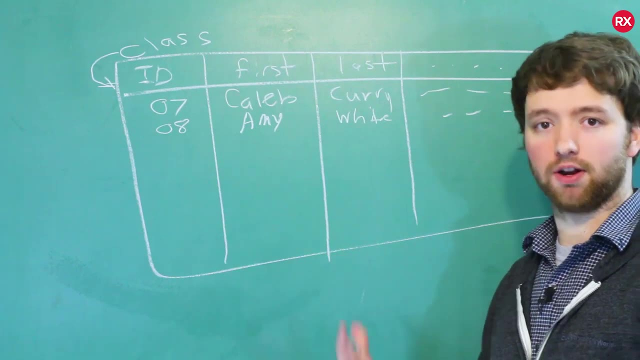 and every time we create a new user, a new object, it's like adding a row. Now, this might be a weird way to think about it, but that definitely helps me because I have a strong database background, if you've watched any other of my videos. So if you've watched my database videos, maybe this is. 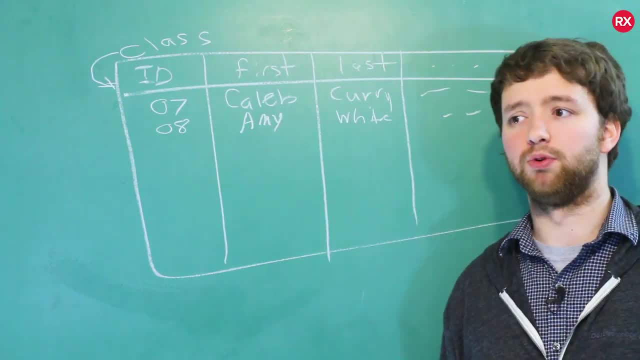 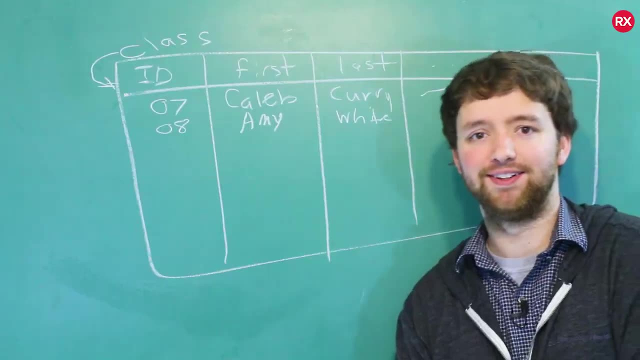 helpful for you guys. Or you might just want to go back to the cookie cutter example, where a class is a cookie cutter and every single cookie we make with that cookie cutter is an object. All right, so what we're going to do now is we're just going to talk about some of the basic concepts. 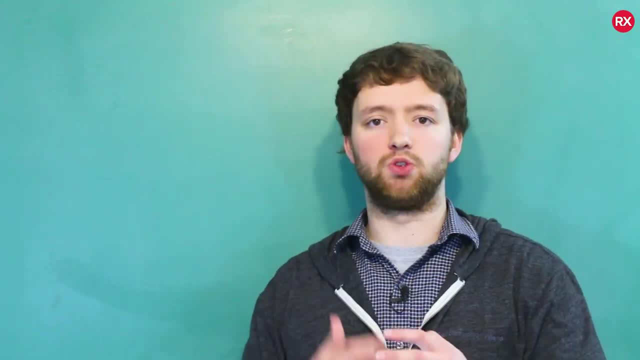 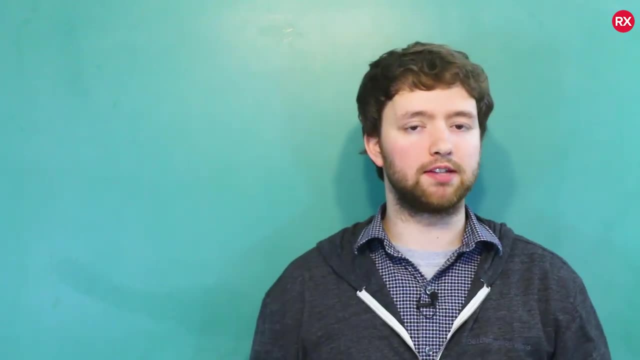 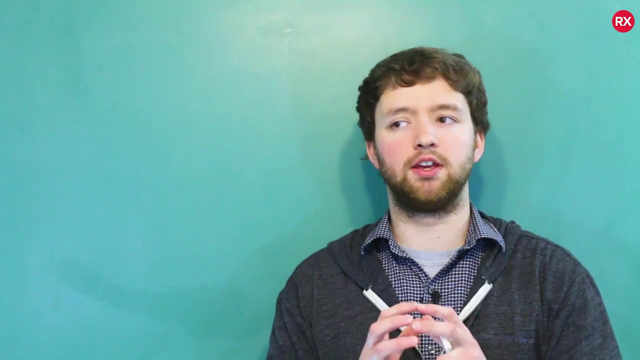 OOP, object oriented programming, before we dive into each one in individual videos. So the first thing we're going to talk about is structs. Structs are very similar to classes, especially in C++. They're almost identical, but by convention, structs are used for smaller things. Maybe coordinates that have an x and a y or a small piece of data where classes are reserved for much larger things. So that's just a convention, but you can do however you want. Once you understand structs, understanding classes is super easy, and vice versa: If you learn classes, first learning structs. 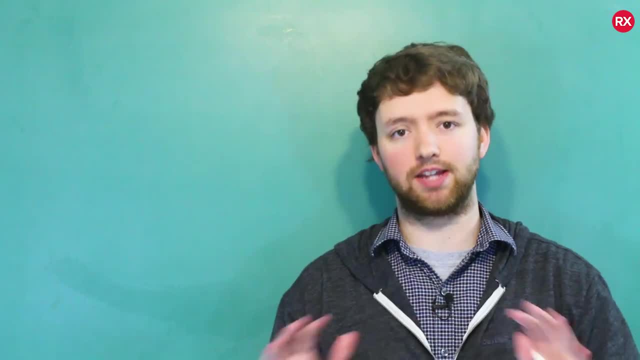 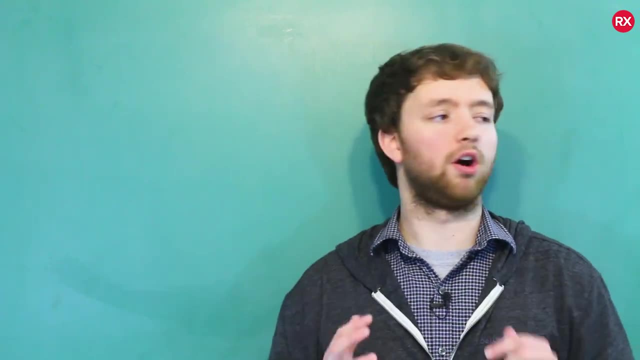 is very, very easy: 15 seconds max. It's almost identical. Other programming languages: that's not entirely gross. Other programming languages: that's not entirely the case. where Onyx quit gagging Other programming languages- that might not be the case. oh my gosh, I'm so annoyed. 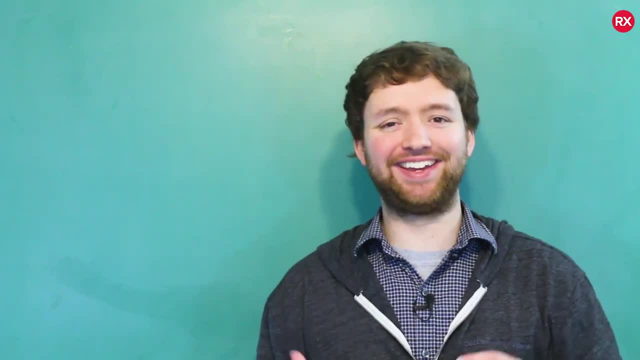 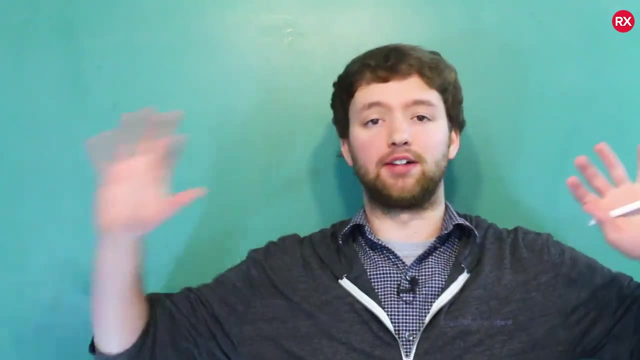 Are you okay? Other programming languages: that might not be the case. gosh, dang it. Other programming languages: that might not be the case. there might be a larger distinction between classes and structs, and that's fine. We're in C++, so I don't know why I keep talking about.